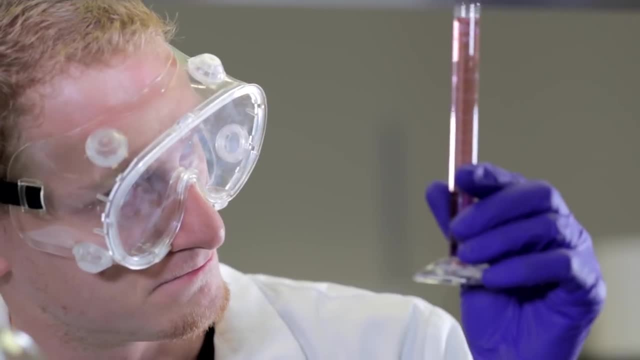 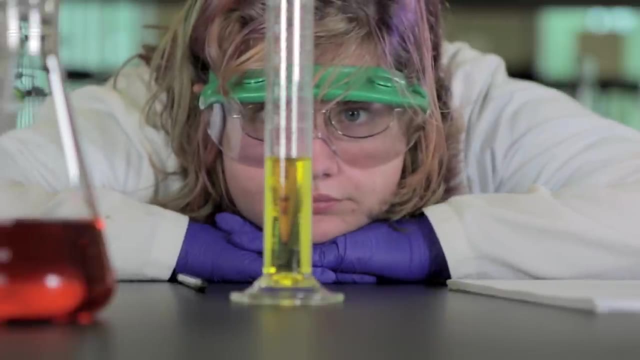 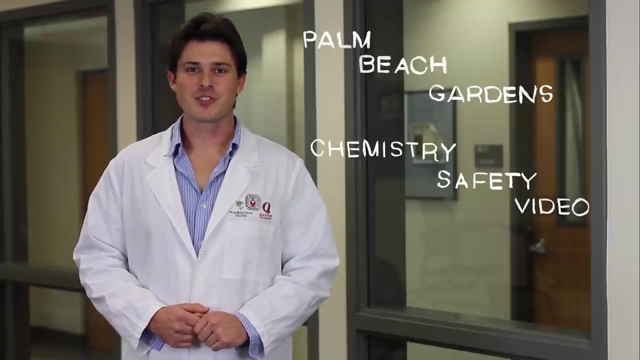 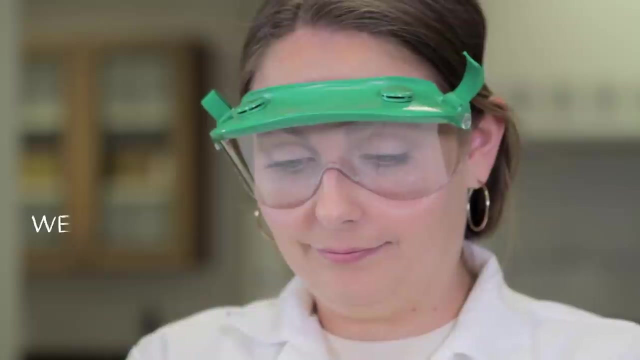 How's it going? My name is Shonska Candy and I'm going over your safety rules at Palm Beach State Chemistry Lab. Make sure you thoroughly read the instructions before starting a lab. Safety goggles are a must. They must be worn in the lab at all times. I would highly advise. 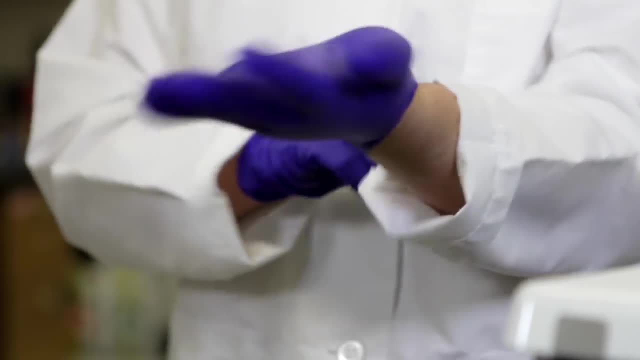 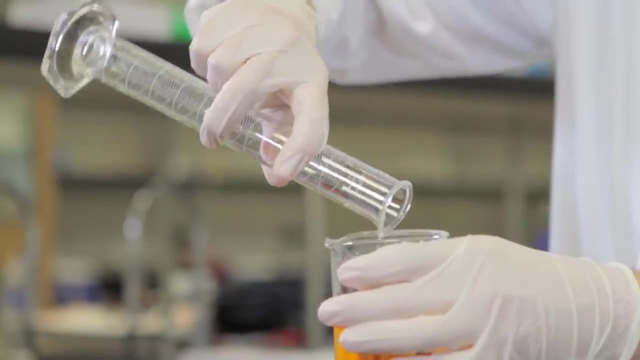 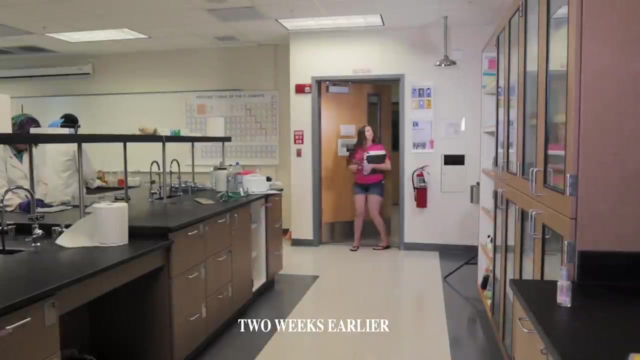 that you also get a lab coat to protect your clothing and, more importantly, to protect your skin. Shoes that cover the top of your feet are very important also, so this goes for the ladies and for the guys that there are no flip-flops allowed in the lab Make. 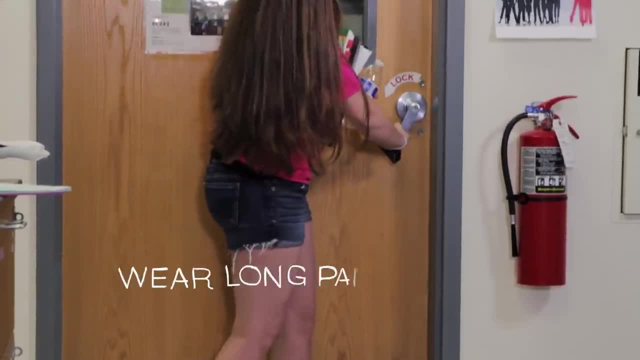 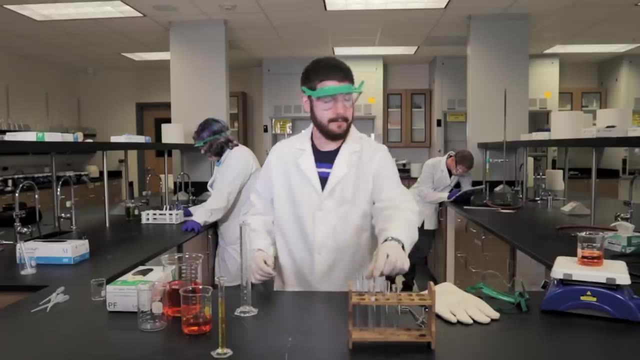 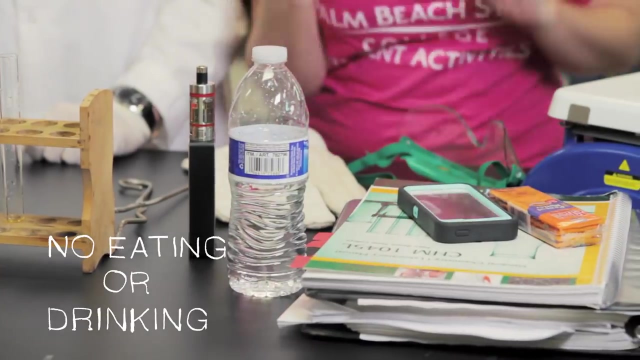 sure that you have long, loose-fitting pants to protect from chemicals also, And, ladies, please remember to wear your hair back. Come on, Come on, It's so late already, Sorry. Make sure that there's no eating or drinking in the lab for your safety, and definitely no smoking. This includes the new electronic. 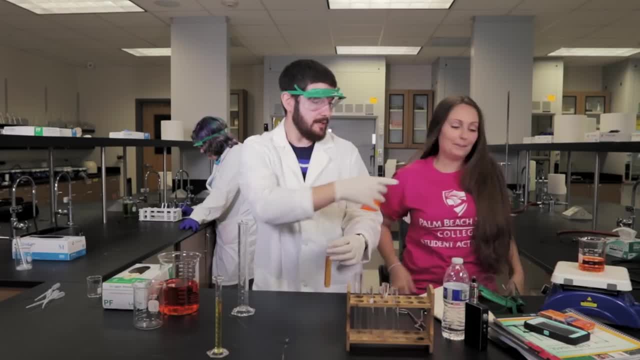 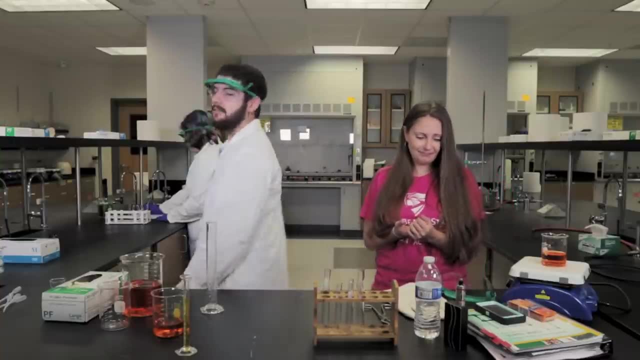 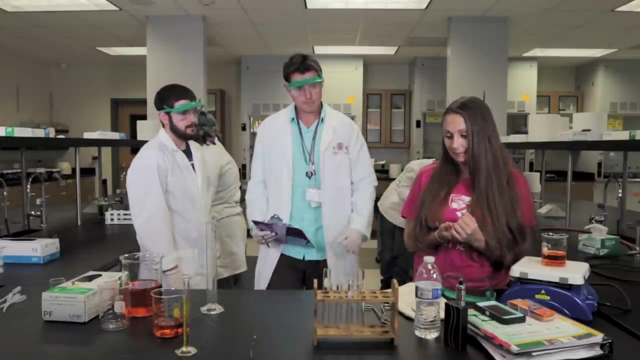 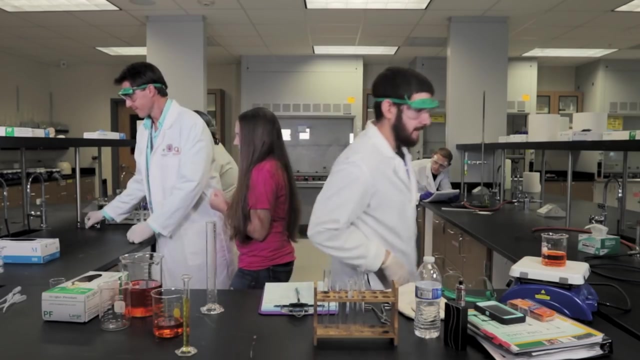 cigarettes. They are not allowed in the lab. What am I doing? Take that off of there. C'mon, Professor, What's wrong? You burned your hand. You burned your hand. Never handle hot objects with your bare hands. You are provided with heat-resistant gloves. 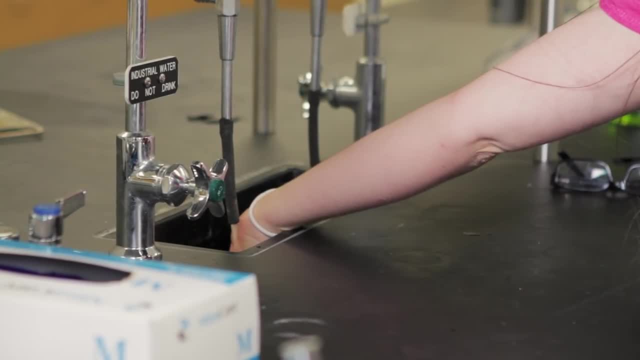 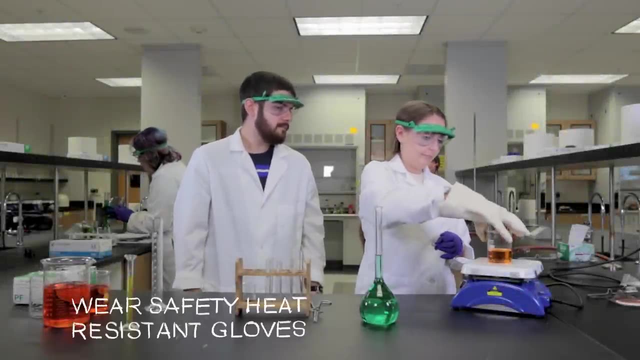 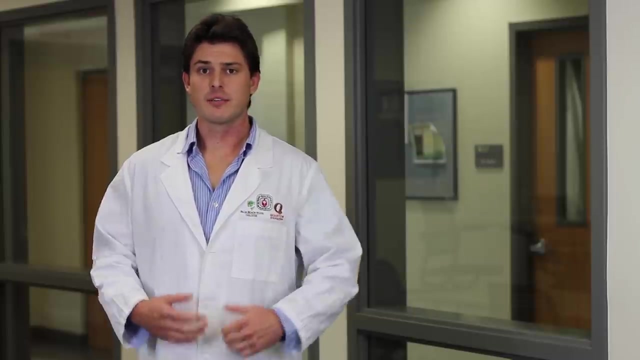 and tongs in the lab. Now, dealing with small burns, immediately go to the sink and rinse. Always remember to wear safety gloves while working in the chemistry lab. Make sure that you familiarize yourself with these different features in the lab in case of an emergency. 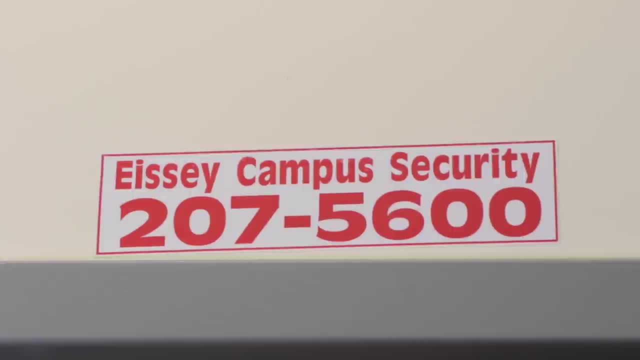 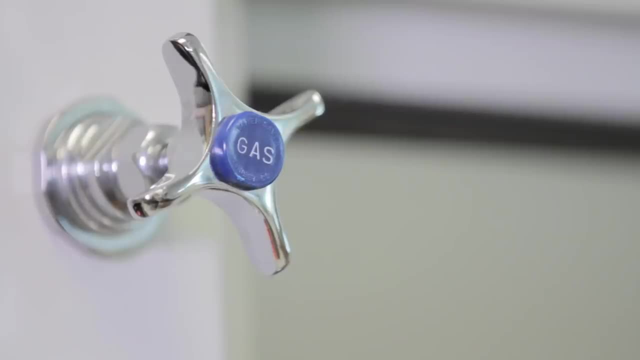 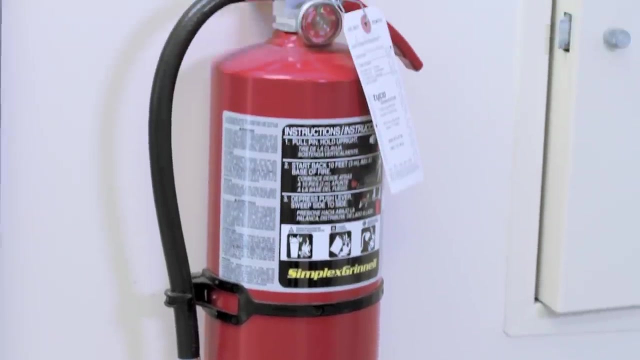 situation. Look around and see where all your safety gloves are, Know where your exits are, Know where your eyewash station is, Know where your shower is your emergency shutoff, your emergency gas shutoff, and familiarize yourself with all the fume hoods. Know where the fire extinguisher is in case of an emergency also. 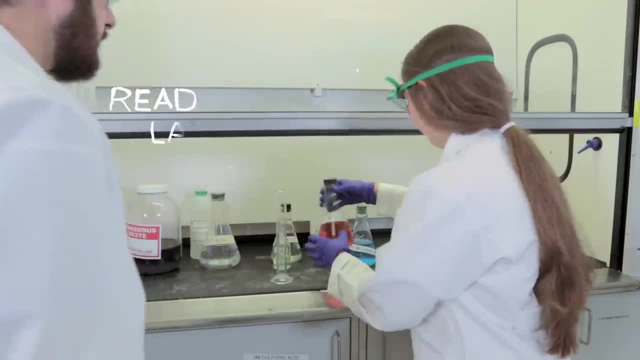 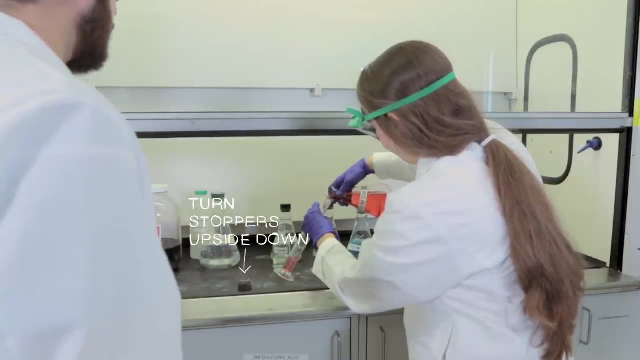 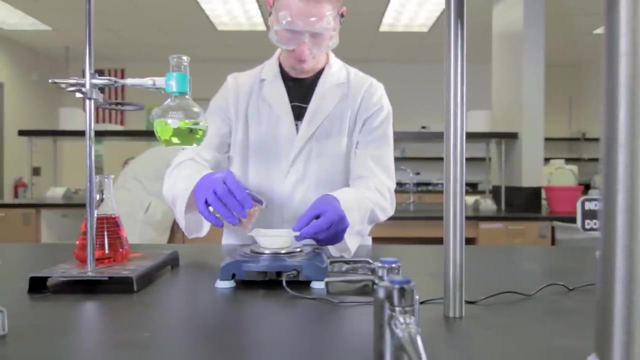 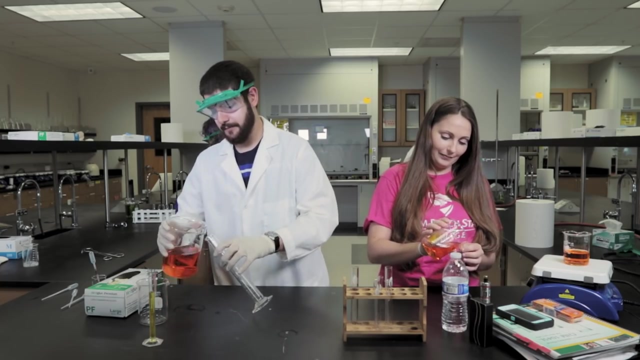 Treat all chemicals as hazardous and make sure to read your labels twice to make sure you have the right chemical. Do not weigh materials directly on the balance pans. Use glassware such as a beaker or a designed way paper. If you cut yourself, immediately rinse the 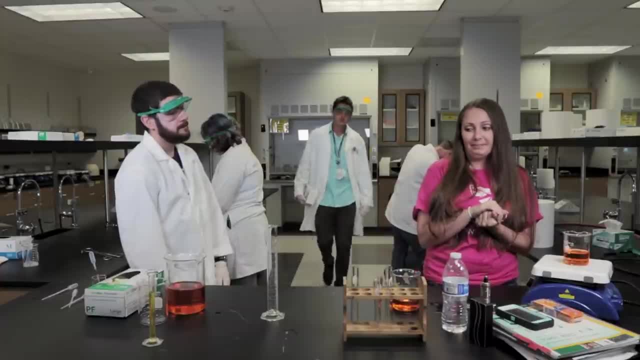 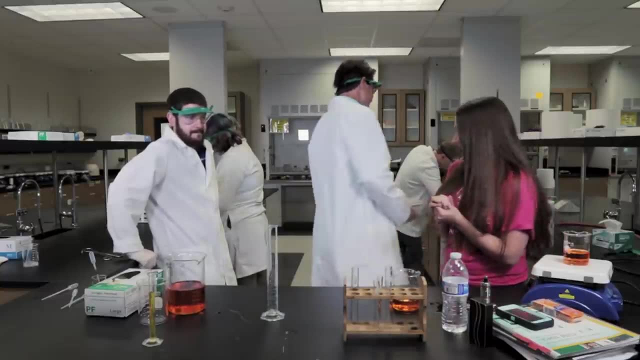 affected area and your instructor will come with a first aid kit. What happened to this one? Is your hand? ok? Oh my gosh, Need to go over this area. The first thing you should do if something breaks in the lab is tell your instructor. 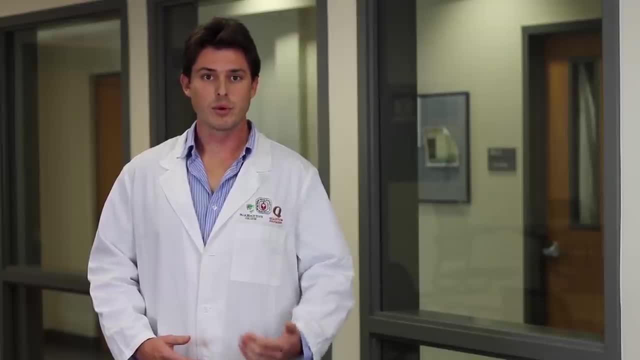 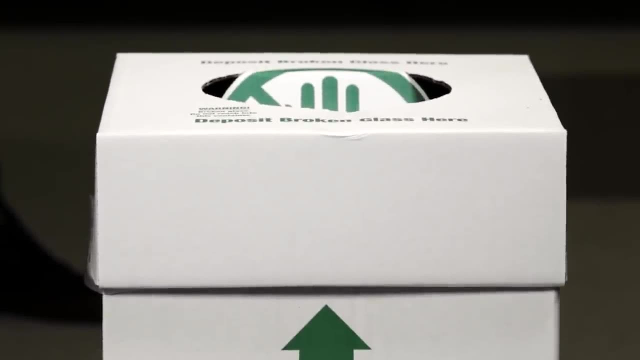 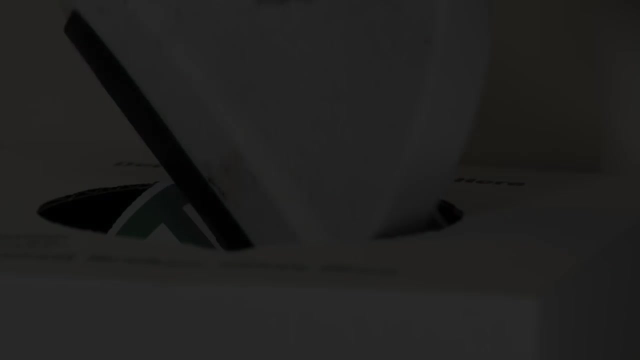 immediately. Your instructor will then guide you where the brooms and dust pans are to handle this broken glassware. Remember: broken glassware only goes in the broken glassware bin. We don't throw paper disposal in it or any other waste in this broken glass disposal. 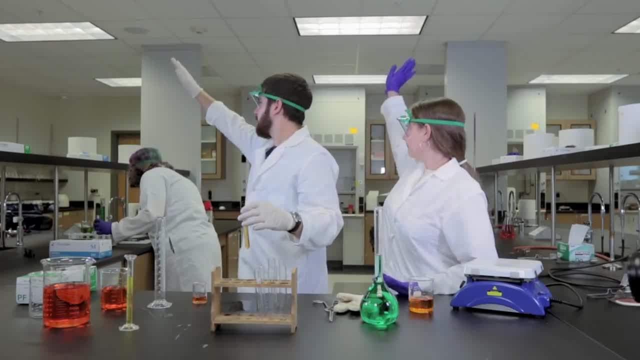 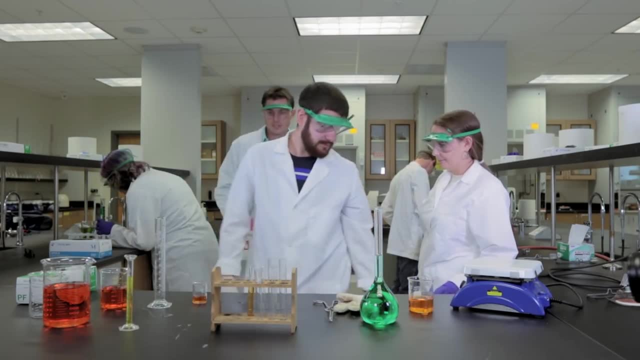 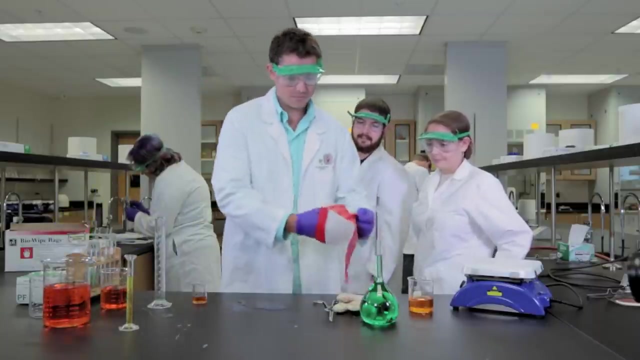 Next, I'd like to go over how to handle a chemical spill. First contact your instructor and let them know that a chemical has been spilled. They will then instruct you how to handle this chemical spill, either using a spill kit or with small spills, possibly using paper towels. 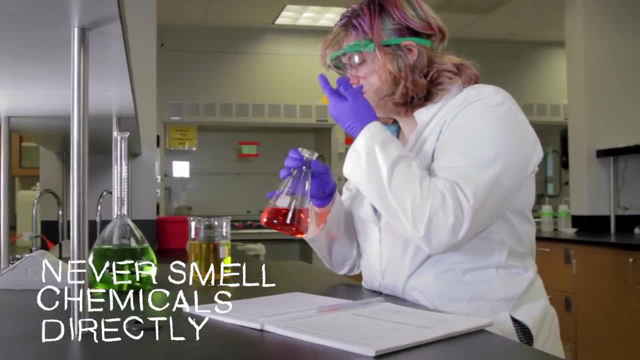 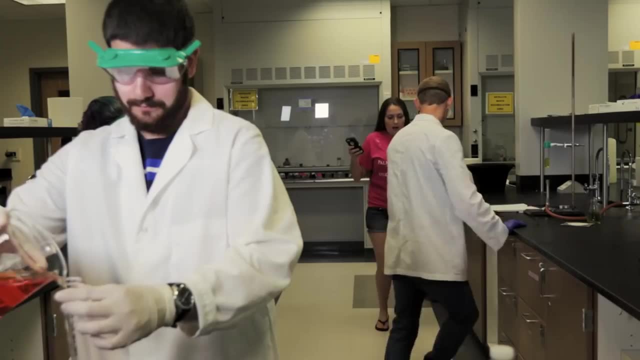 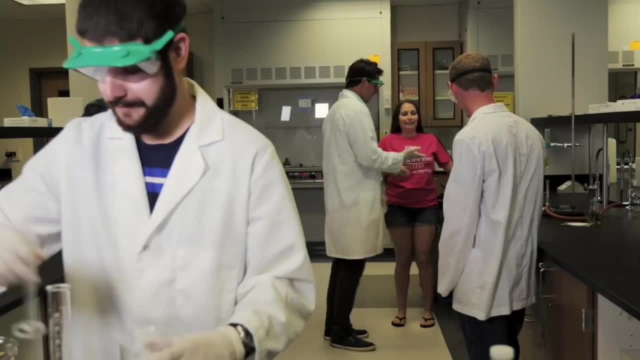 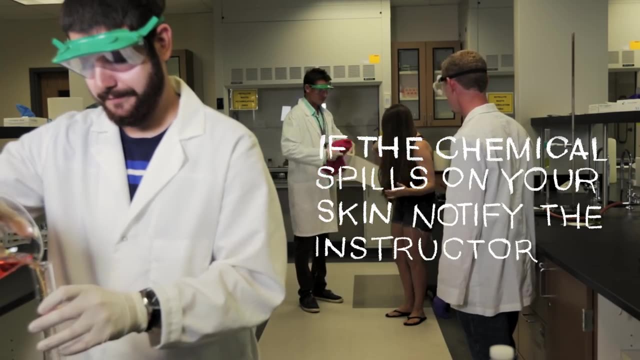 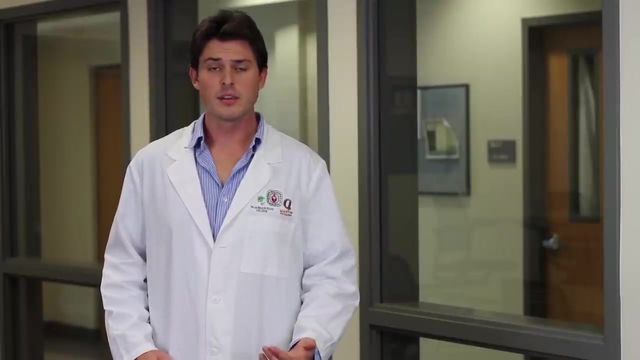 Oh my gosh, All right, we have to move the clothes immediately. Turn on the comb. If spills occur on your clothing, you must first remove the affected area and then rinse immediately, Depending on the size of the spill. a small spill can be rinsed in the sink and a larger